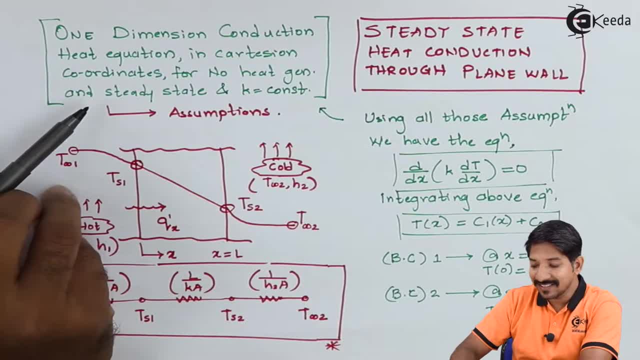 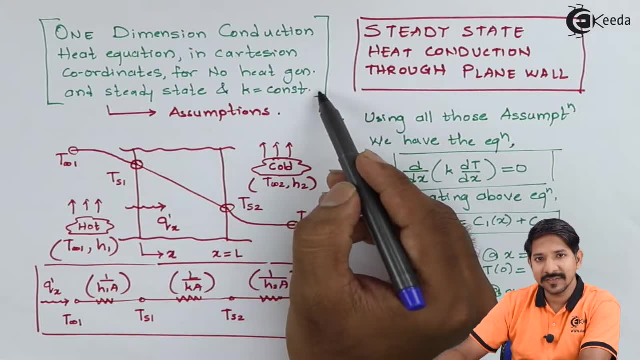 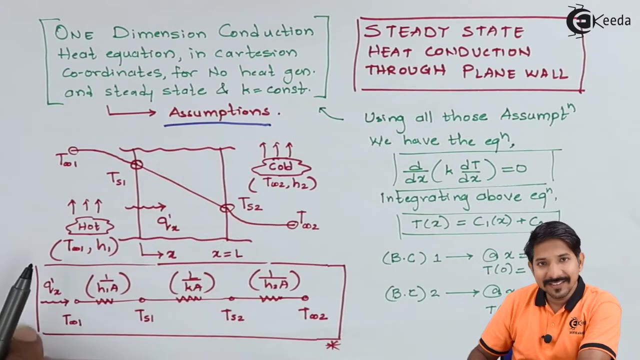 is no heat generation and there is a steady state heat transfer. The last one is: we will assume that the value of K, that is, the thermal conductivity, is constant throughout the material. These are my set of assumptions. Now let us consider that there is a small wall to the left, that the temperature Ts 1, and to the right there is. 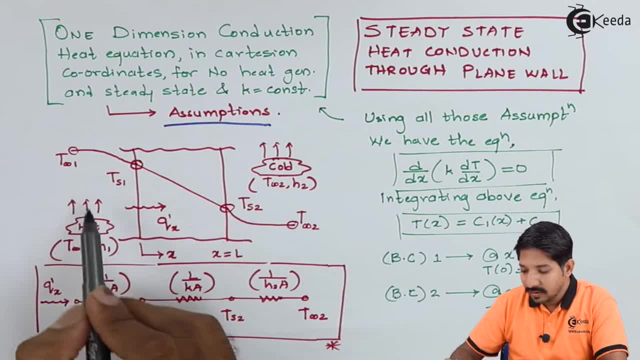 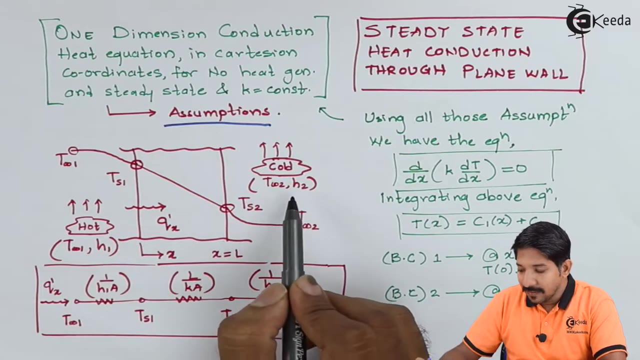 a temperature Ts 2.. There is a hot fluid flowing to the left hand side of the wall and the cold fluid flowing to the right side of the wall. The temperature of hot fluid is T, infinity 1. rate. the heat transfer coefficient is h1 over here. Similarly the temperature of cold fluid. 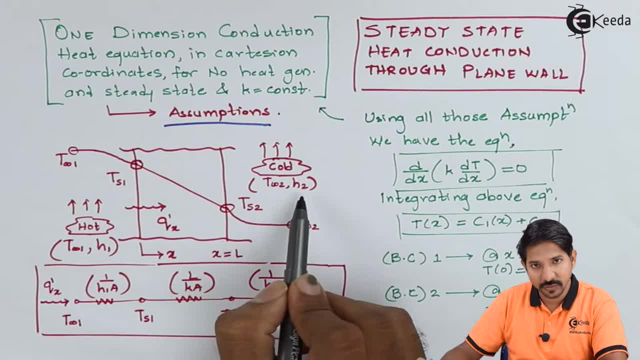 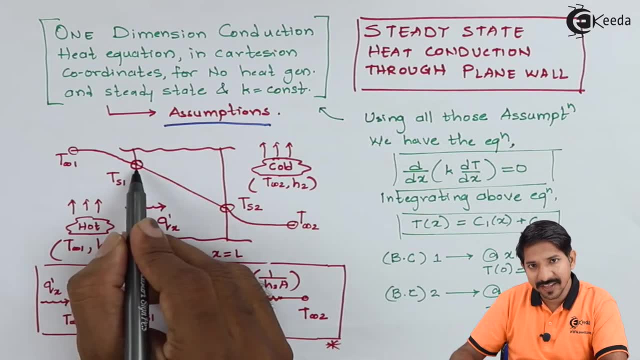 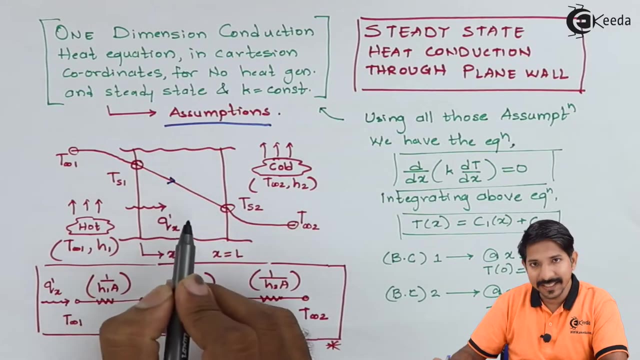 is, let's say, T infinity 2, and the heat transfer coefficient is h2.. So obviously there is a drop from Ts1, that is the surface temperature, to the left hand side of the wall, to Ts2, which is the surface temperature of the right hand side of the wall. Now this drop will be linear. 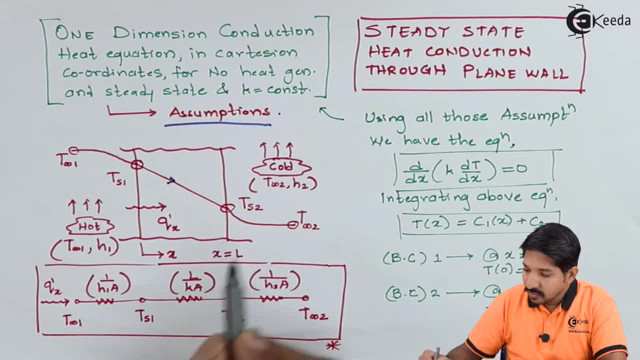 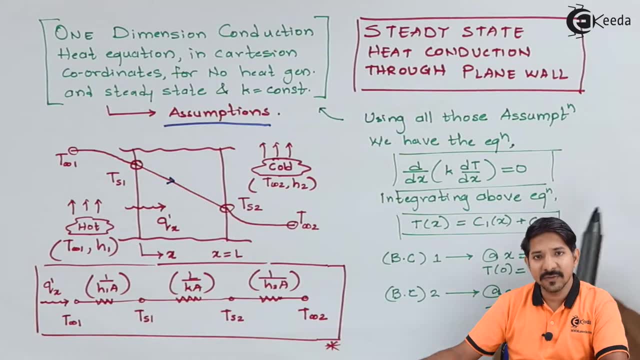 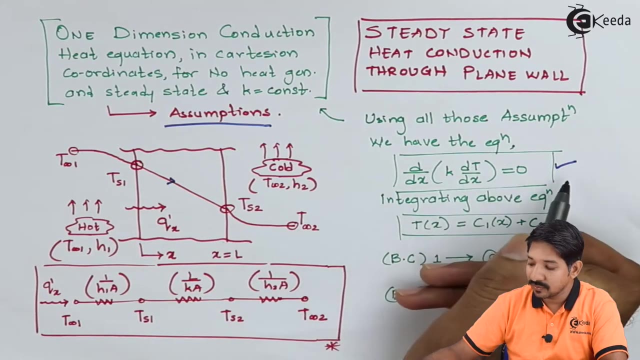 Why we will see later. So in this case, with all these assumptions and with the general equation that we derived previously, We will left with this equation, that is d by dx k, dt by dx equal to zero. Now, if I integrate it twice, I shall get: 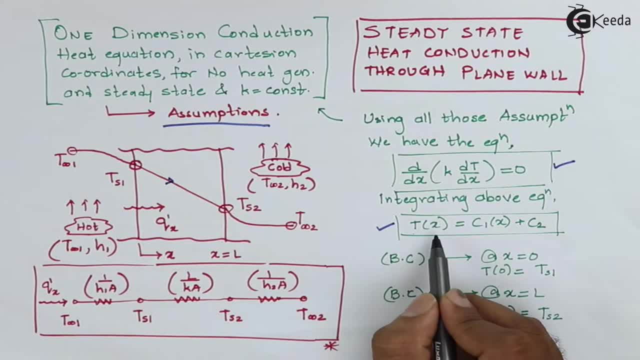 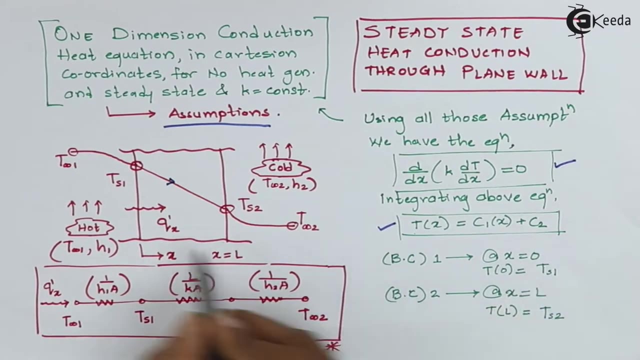 equation something like this, That is, T, which is a function of x, is equal to C1x plus C2.. Now, since two constants, we need two boundary conditions. As we had seen previously, the boundary condition one will be at x equal to zero. So see here, as we had seen previously, the boundary condition. 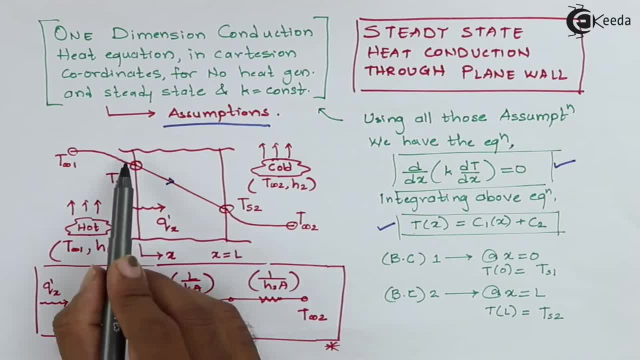 one that is at x equal to zero means at the left hand side surface of the wall the temperature is T. So that makes my boundary condition one: at x equals to zero t. Now, zero is at x equals to zero. Temperature is T. Similarly the boundary condition. 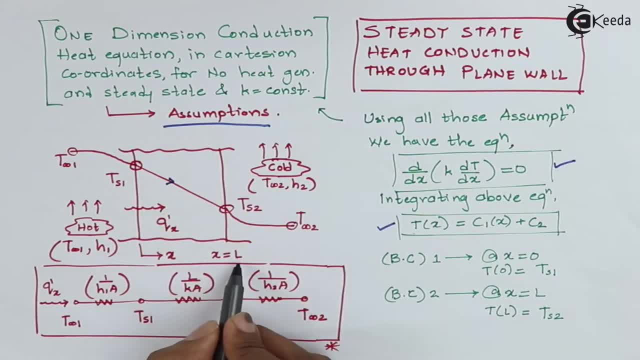 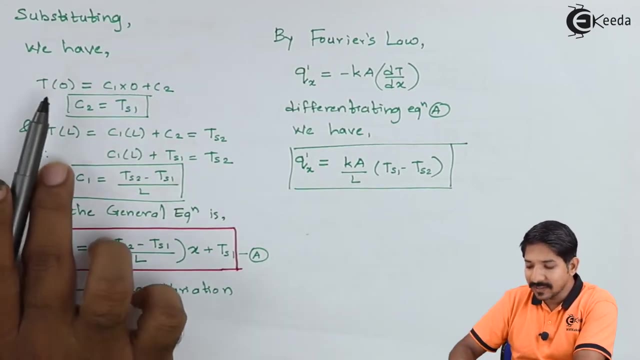 two will be on the right hand side. when the value of x equals to L, my temperature is T, So that makes my second boundary condition. Now I need to put the first and second boundary condition in the general solution over here. If I substitute the same, I shall get equation. 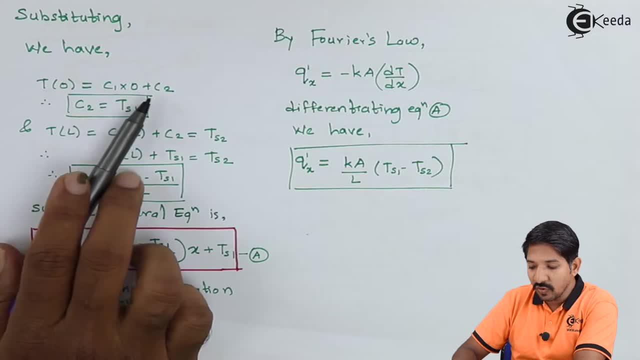 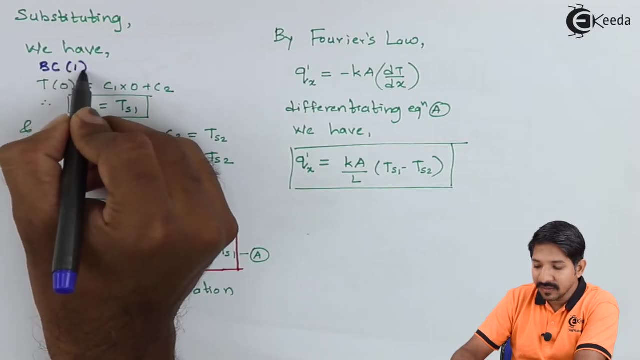 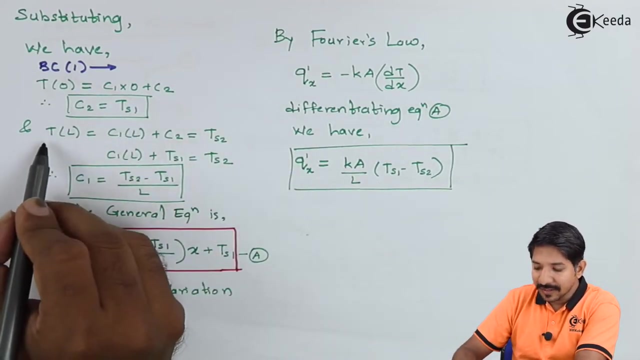 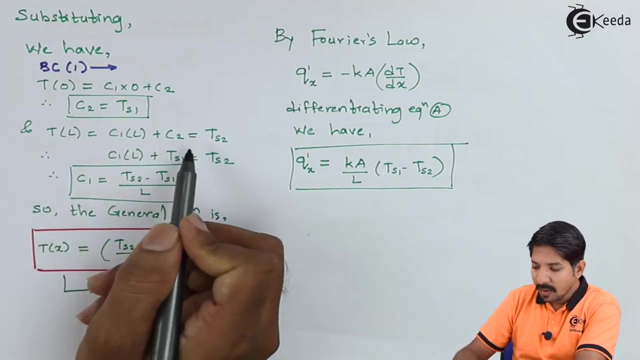 like T of 0, which is equal to C1, into 0 plus C2.. Now here I have substituted the first boundary condition, So I can write: the boundary condition 1 will yield me C2 equal to TS1.. Similarly, with the second boundary condition, if I put, then my equation become T of L equal to C1, L plus C2. 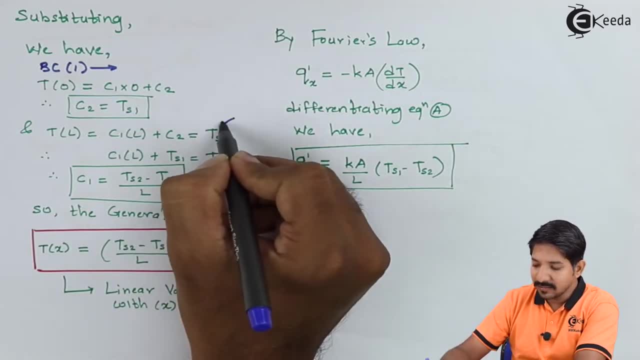 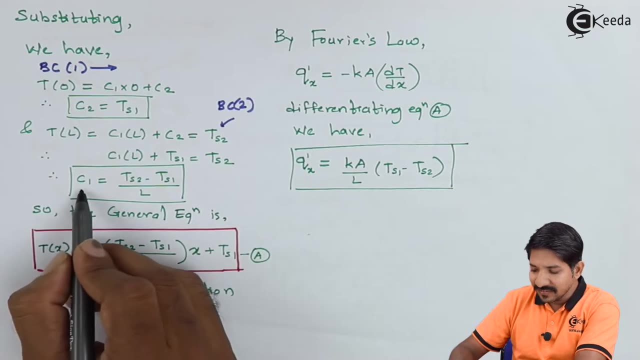 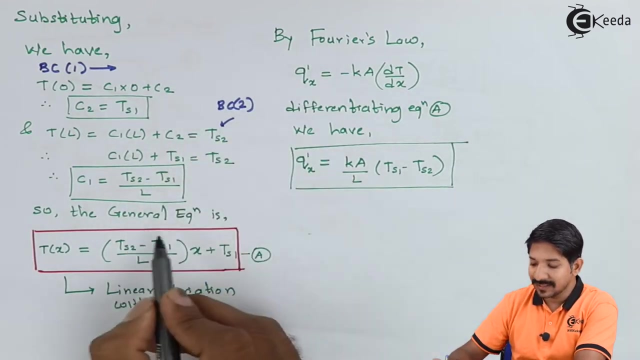 which is equal to TS2.. So now, this is nothing but my second boundary condition. So if I start solving, I shall get the value of C1 as TS2 minus TS1 upon L. Now, these two constants we are going to put in the general solution. So finally, my equation. 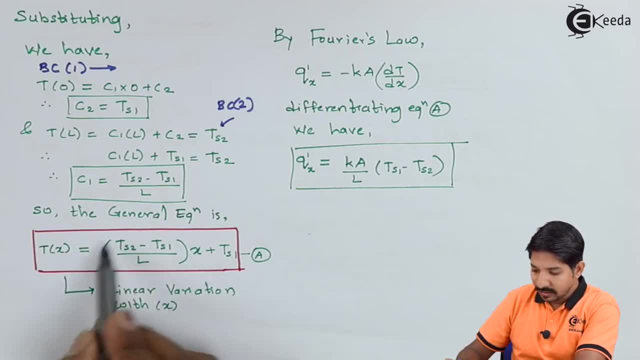 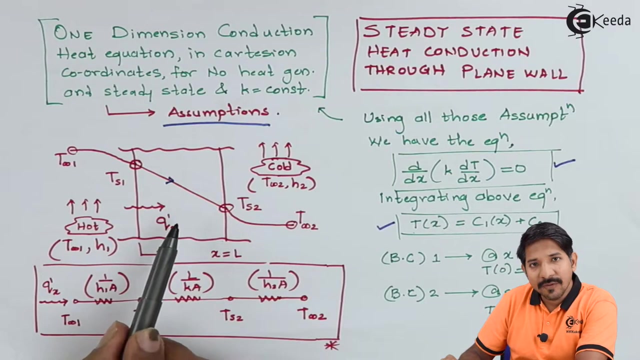 will become: T of X is equal to C1, that is, TS2 minus TS1 upon L into X. So I am giving this as equation number 1.. See, here we can see that the temperature depends linearly on the dimension X, because the power of X is 1.. That is what I was talking about. 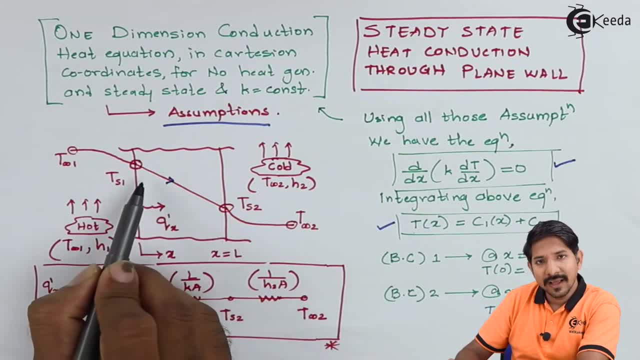 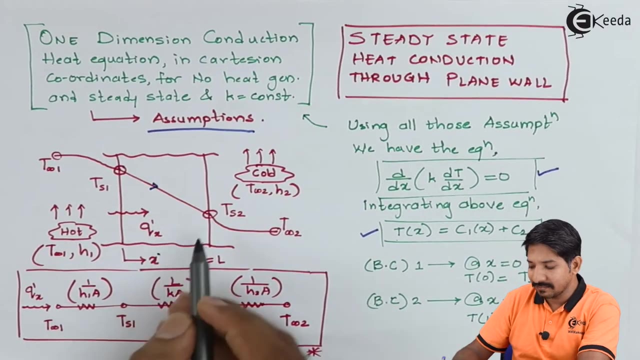 See, I can join this two point by any means. I can join this linearly or some parabolic curve or some cubic curve, But I need to join this linearly because my temperature in this case depends linearly on dimension X. So this, here we get the temperature distribution. 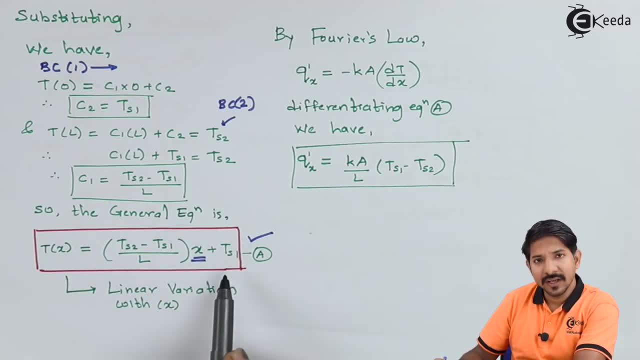 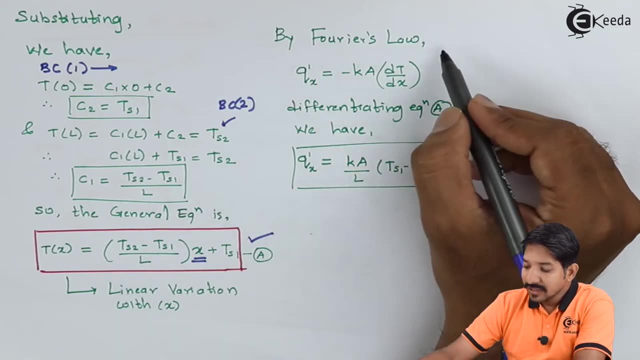 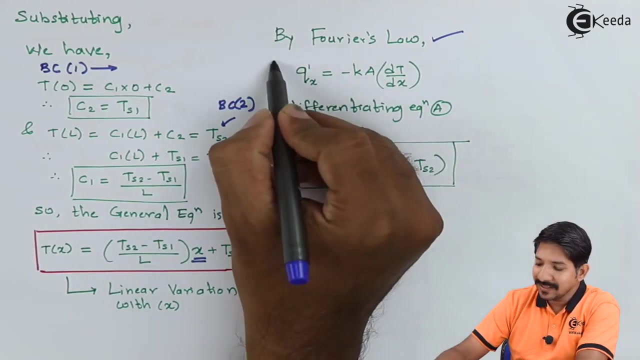 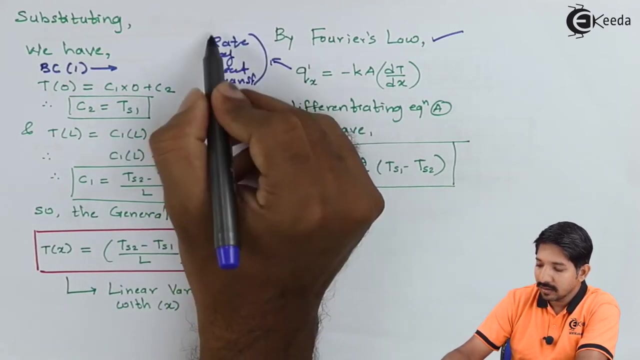 in case of steady-state heat transfer. So this equation talks about the temperature distribution in our case. Now let us see if I use the Fourier's equation, which is Q dash of X, where Q dash is nothing but the rate of heat transfer, which is given as minus K. 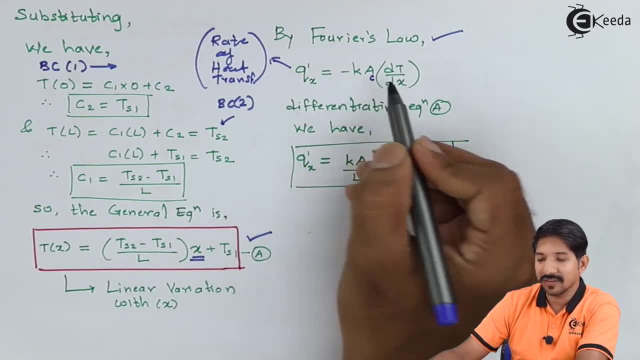 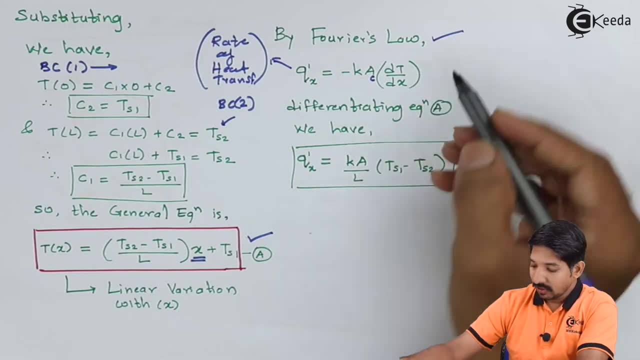 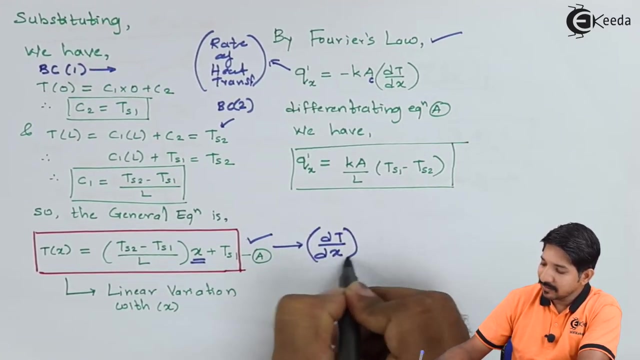 A DT by DX, Now A. here is the cross-sectional area. If I differentiate this equation with respect to X, I can find the DT by DX here. See my differentiation here will yield me: DT by DX is equal to 0.. So see, only the first parameter is having the parameter X over here. See, if I differentiate. 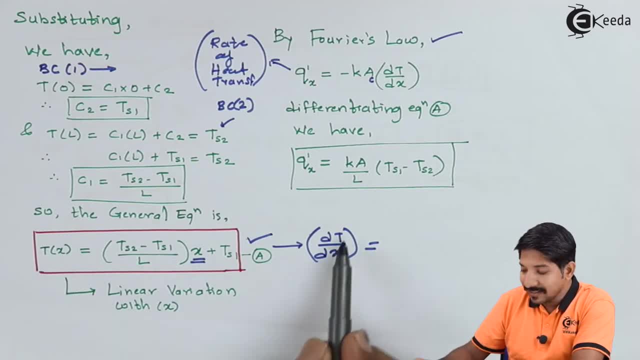 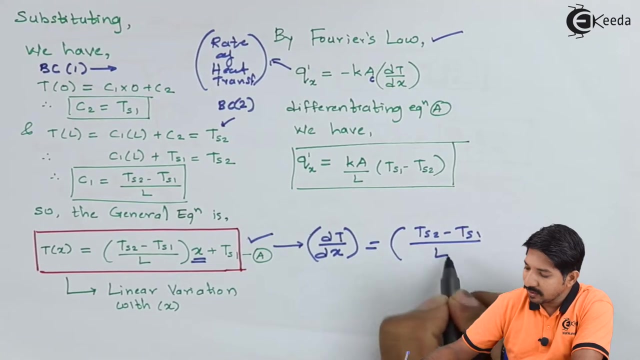 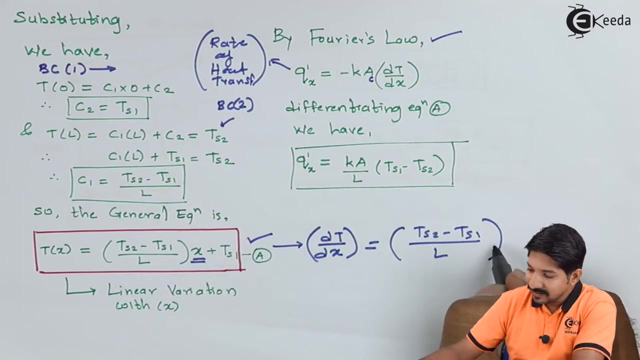 this temperature T with respect to X, DT by DX, then I shall find: see, here only the first parameter is having variable X. So the differential will only give me T S2 minus T S1 upon L. See, this will be constant. So if I differentiate this I shall get 0 over here. Now this is: 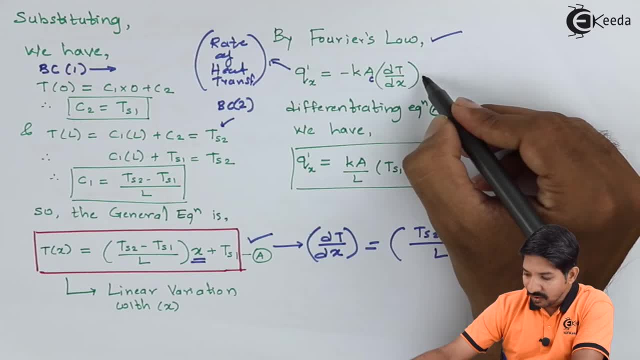 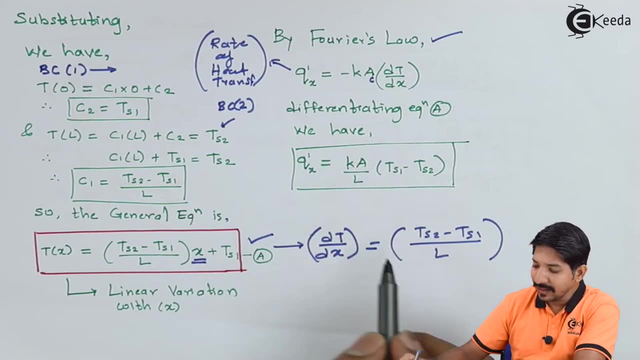 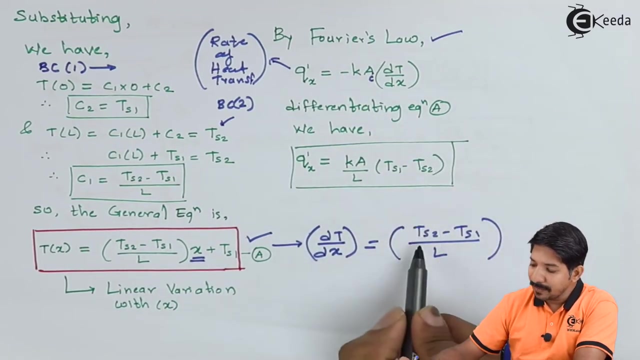 what I have put in this main equation. Then what will I have? I will have Q, dash of X is equal to this K into A, which I have written over here upon L. Now this L will come over here and then, to compensate the negative sign, what I will do? I will simply change my temperatures. 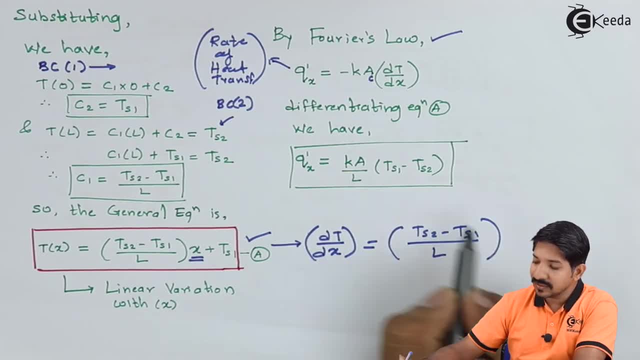 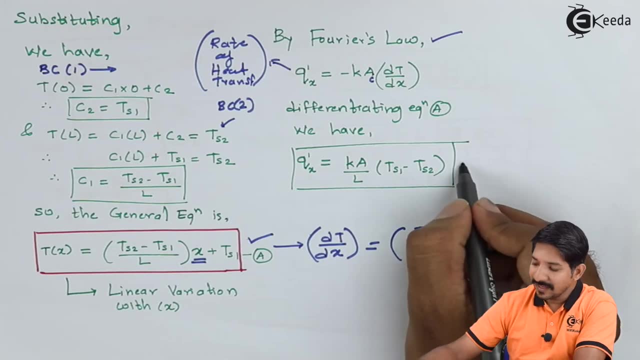 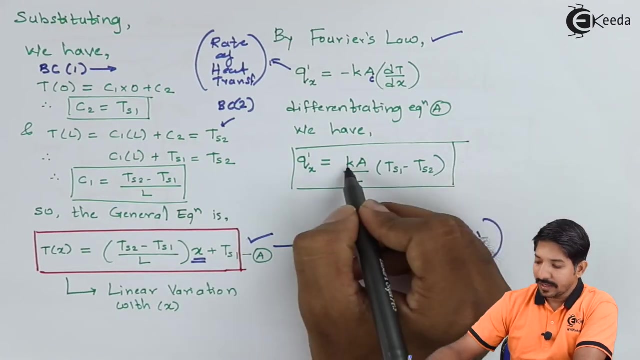 See here, with the differential, we are getting T S2 minus T S1.. To negate this negative sign, I will write this as T S1 minus T S2.. So finally, we will get the value of heat transfer rate, in this case as T S1 minus T S2, into. 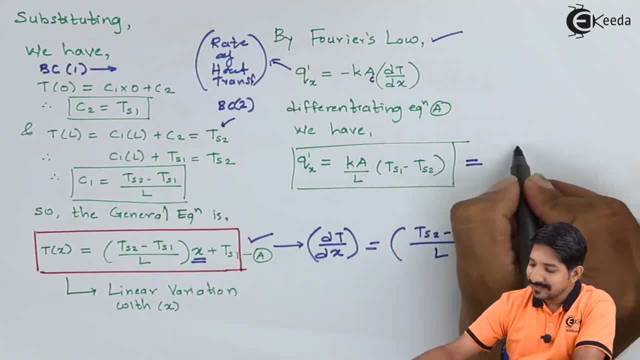 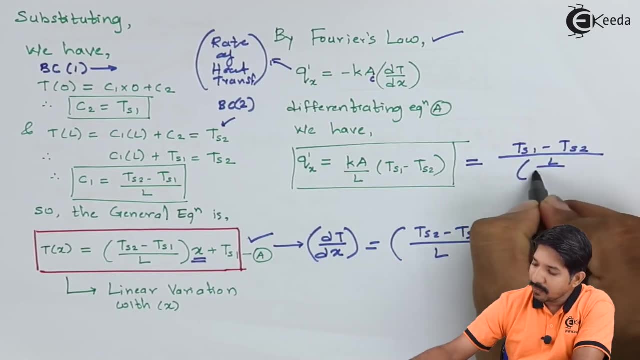 K upon L. As we had seen previously, this can also be written as T? S1 minus T S2 upon L upon K A. Now, this L upon K A is nothing but your thermal resistance in case of conduction. See now the derivation that we had for the. 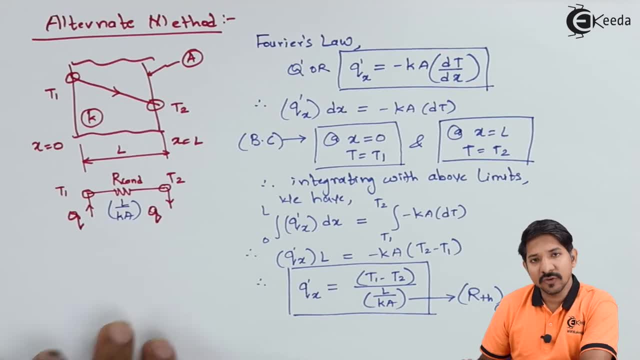 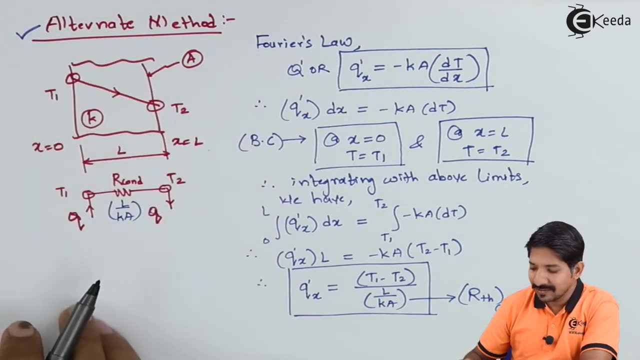 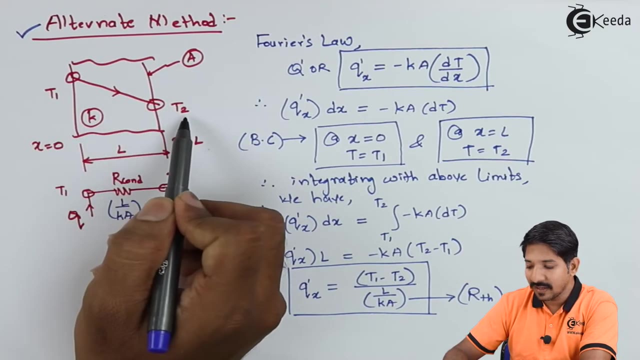 heat transfer rate in case of single wall can also be done without the use of general equation. So let us see the alternate method for the same Again what we have done. we have considered a wall where the temperature to the left hand side is T1. to the right hand side, we have 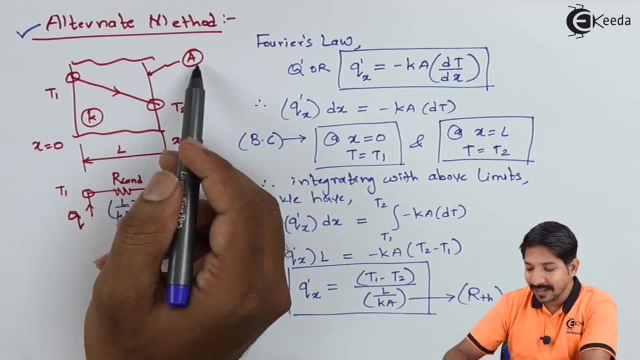 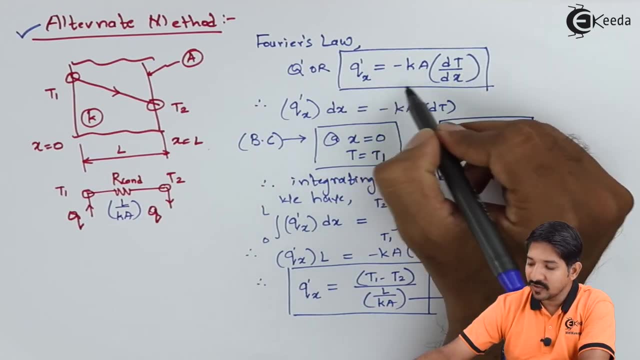 got T2.. The conductivity is K, The cross section area is A and the length is L. So here I will simply write down the Fourier's law, which is Q dash of X equal to minus K dT by dA. Now let us look at the Fourier's law, The Q dash of X. 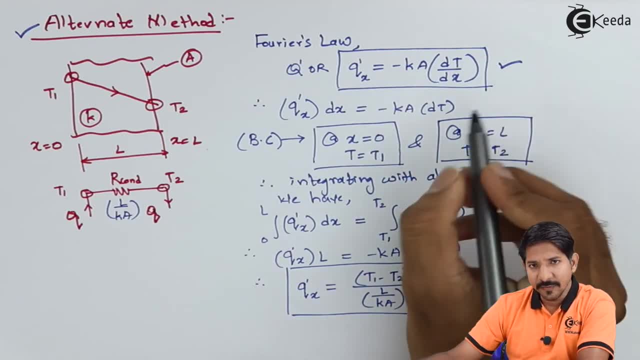 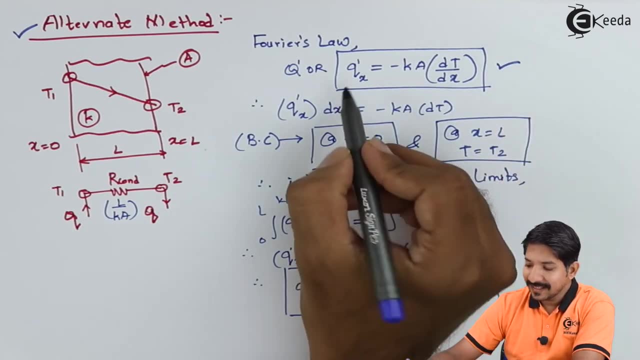 is equal to minus K dT by x. Now here we will simply go for the rearrangement of the variables. So with the help of Fourier's Law we can say that Q dash of X is equal to minus K dT by dX. Now here we will simply. 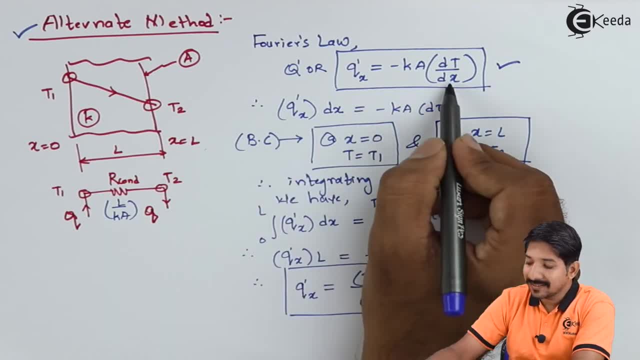 go for the rearrangement of the variables. So let us take this dX to the left hand side of the equal to sine, then we will have Q dash of x into d x, So 되고, let's take this to the left hand side of the equal to sine, then we will have to cry into the Governor: X into D X minus T Berry, equal to D x. sorry. 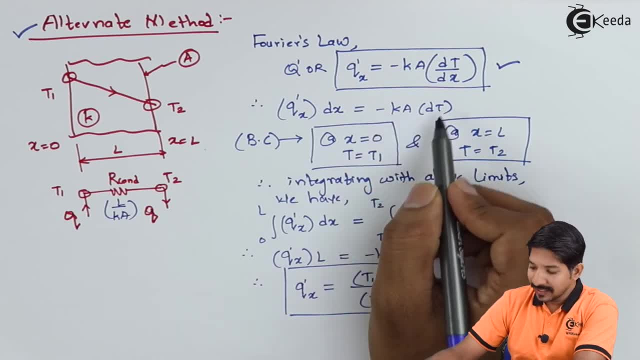 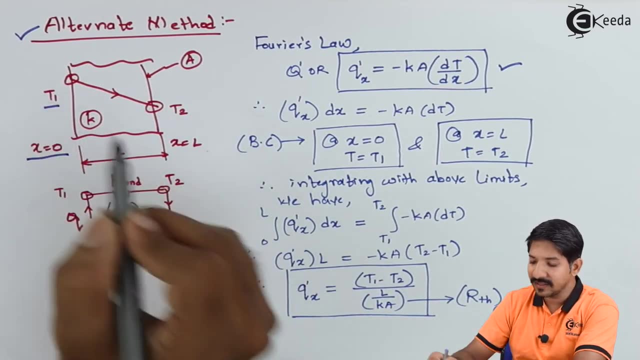 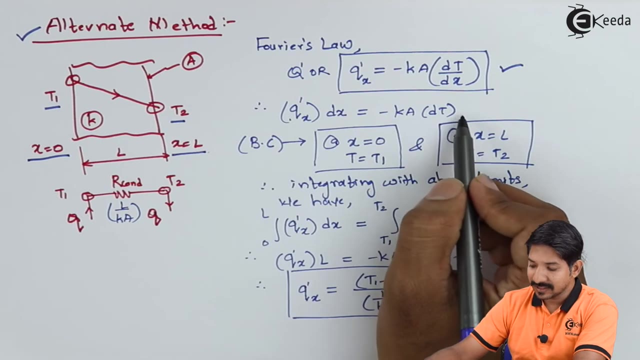 is equal to minus K ADT. now, again, using the same boundary conditions which we have seen previously, that is, at x equal to 0, my temperature is T1, and at x equal to L, my temperature is T2. if I use these two boundary condition and if I integrate this equation, I shall get something. 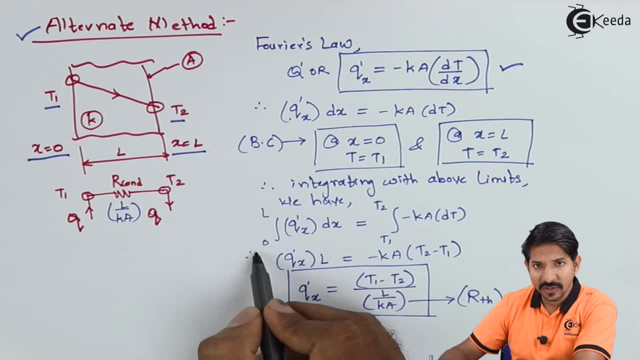 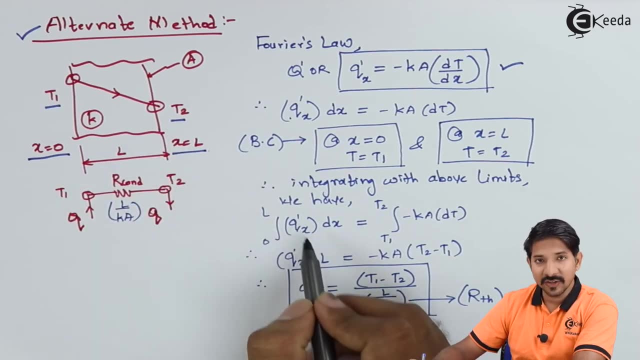 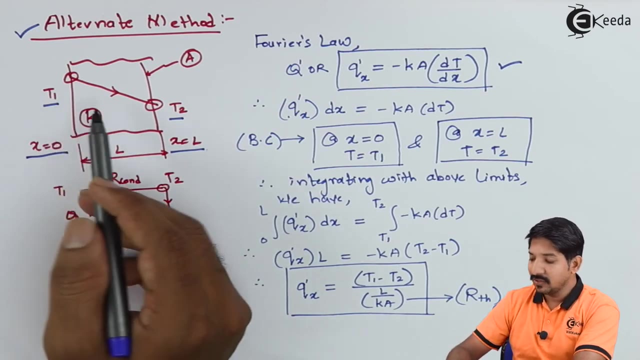 like this: that is integral 0 to L. so why 0 to L? because my x is standing from 0 to L. Q dash of x, DX is equal to integral, now corresponding to x equal to 0. my temperature was T1, so hence my lower limit of integral will be T1 over here and then the higher limit of integral. 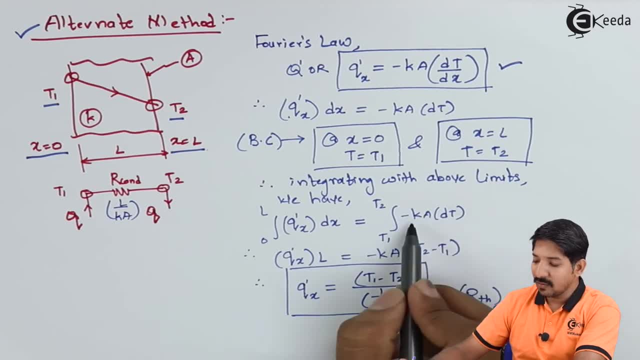 will be T2 over here and in the bracket we have minus K ADT. so if I go for normal procedure of integration, then I can finally say that we will again get the value of Q. dash of x is equal to even minus T2 upon L, upon K a. 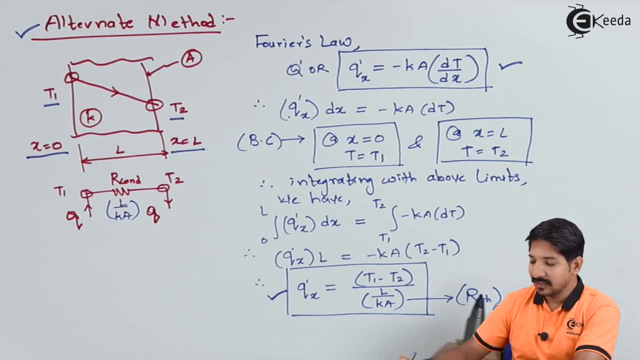 So Well, Well, So, which is nothing but the thermal resistance of the conduction. Now, this is the same equation we had got previously, But in the previous case we could have found the temperature distribution also from the main general solution. Here we will only get the heat transfer rate. 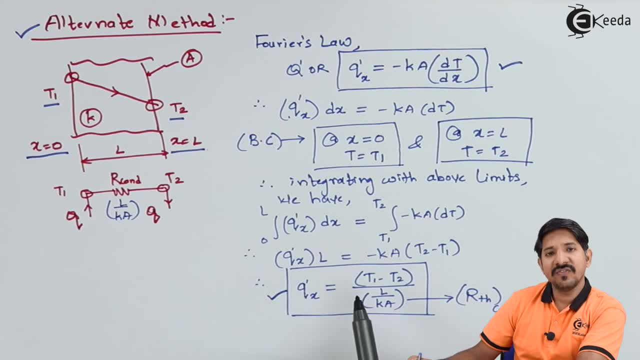 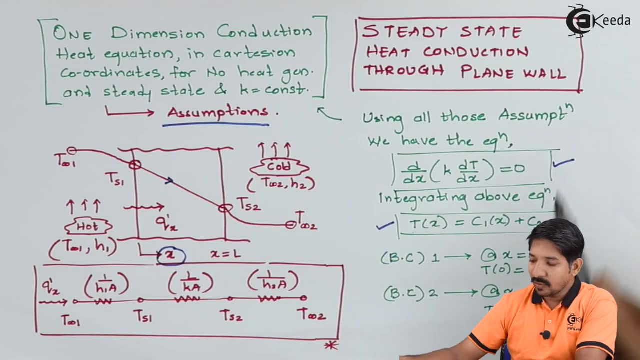 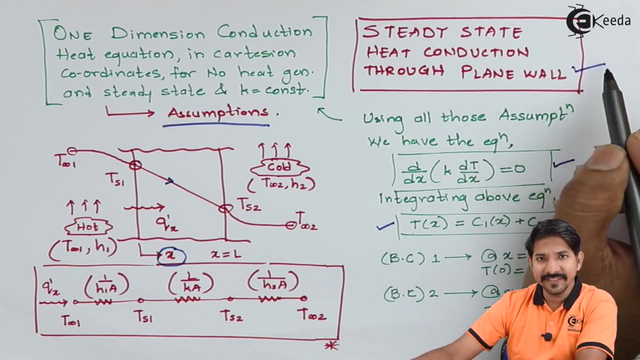 You can choose the either method, But the first method is more equipped to find the temperature distribution for any given case. That is it in this topic. Here we have discussed basically the steady state heat conduction through plane wall And we have tried to derive. 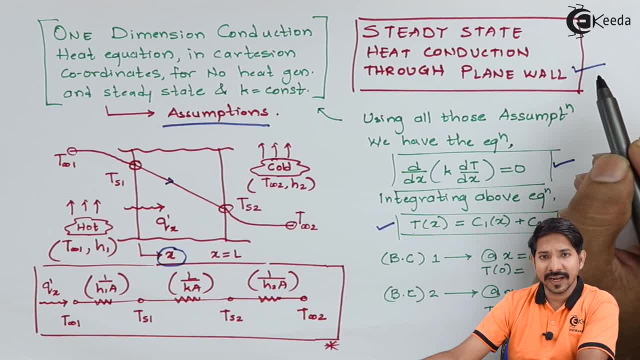 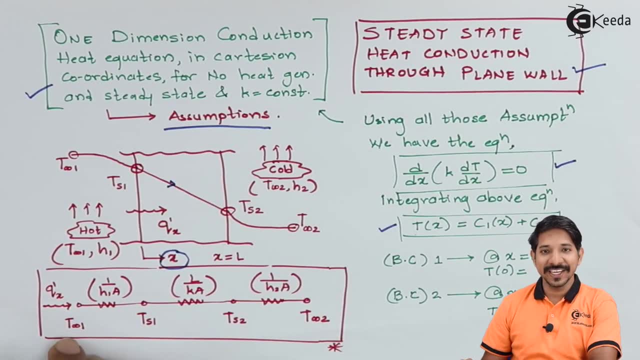 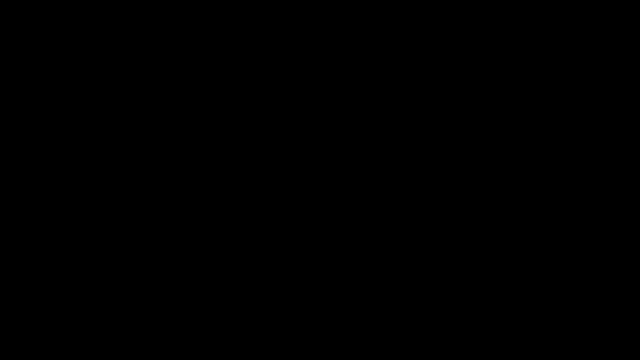 the temperature distribution and heat transfer rate in this case. with these many assumptions, Thank you for watching this video. Please stay tuned with eKIDA. Please subscribe to eKIDA. Thank you, Thank you.